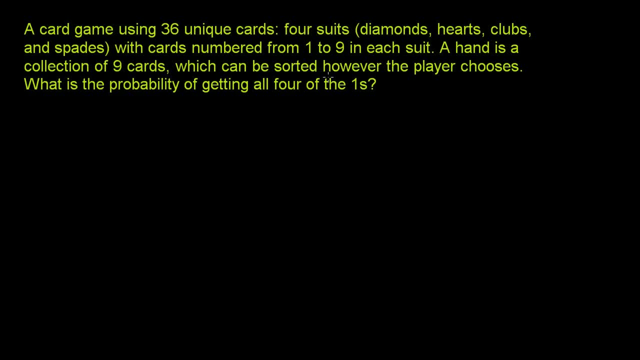 A hand is a collection of nine cards which can be sorted however the player chooses. So they're essentially telling us that order does not matter. What is the probability of getting all four of the ones? So they want to know the probability of getting all. 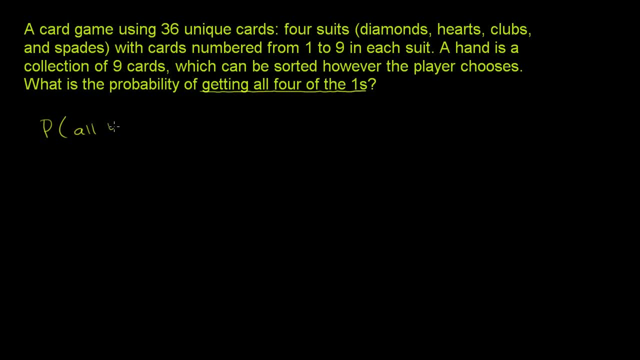 four of the ones, So all four ones in my hand of nine. Now this is kind of daunting. at first You're like gee, I have nine cards and I'm taking them out of 36, I have to figure out how do I get all of the ones. 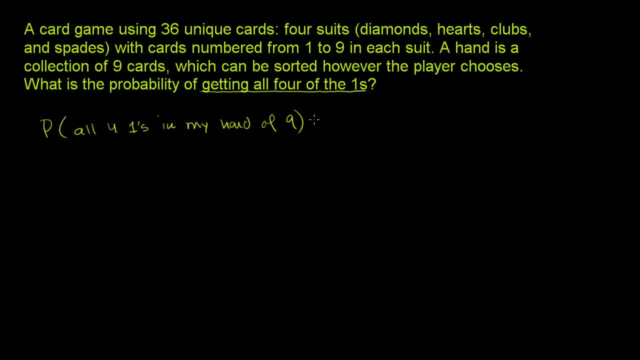 But if we think about it just in very simple terms, all a probability is saying Is the number of events, or I guess you could say the number of ways in which this action or this event happens. So this is what the definition of the probability is. 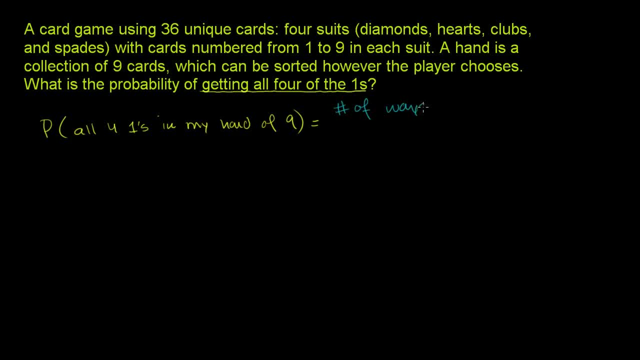 It's going to be the number of ways in which event can happen, And when we talk about the event, we're talking about having all four ones in my hand. That's the event, And all of these different ways. That's sometimes called the event space. 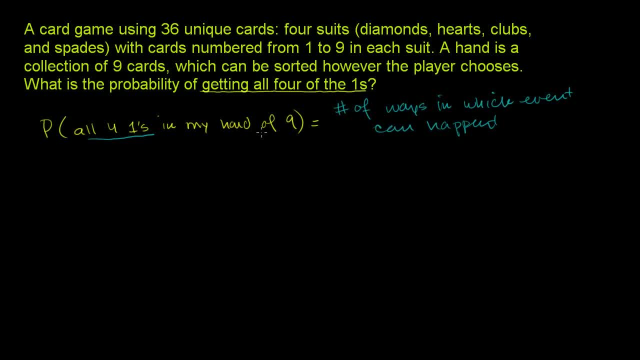 But we actually want to count how many ways that if I get a hand of nine- picking from 36, that I can get the four ones in it. so this is the number of ways in which my event can happen and we want to divide that into all of the 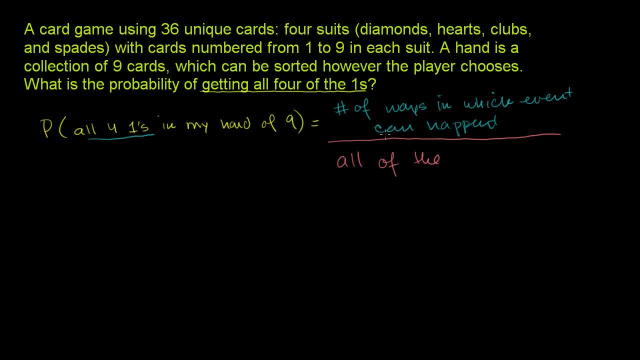 possibilities, all of the, or maybe I should write it this way- the total number of hands that I can get. So the numerator in blue is the number of hands where I have, or the number of different hands where I have, the four ones and we're dividing it to divide the. 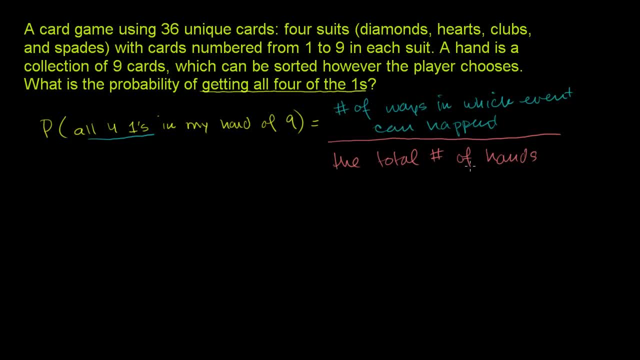 total number of hands. Now, let's figure out the total number of hands first, because at some level this might be more intuitive, and we've actually done this before. Now, the total number of hands. we're picking nine cards and we're picking them from a set of 36 unique cards. 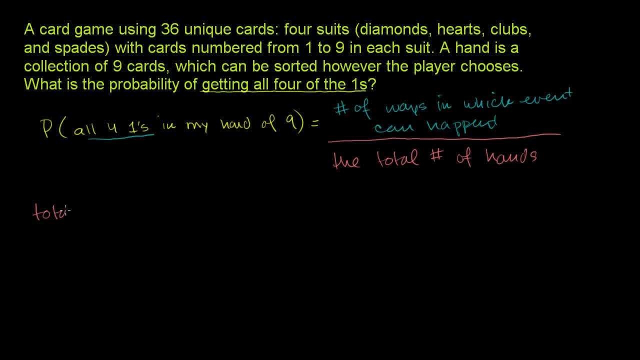 And we've done this many, many times. so let me write this: Total number, Number of hands or total number of possible hands. That's equal to. you can imagine you have nine cards to pick from. the first card you pick is going to be one of 36. 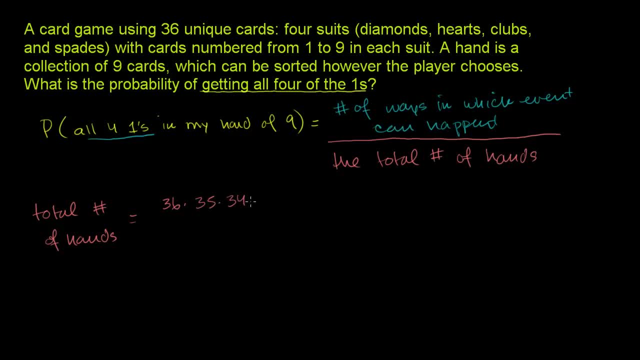 cards, then the next one's going to be one of 35,, then the next one's going to be one of 34,, 33,, 32,, 31.. We're going to do this nine times: One, two, three, four, five, six, seven, eight and nine. 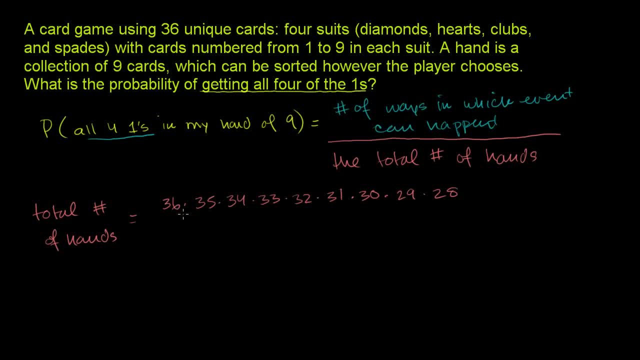 So that would That would. That would be the total number of hands if order mattered. But we know, and we've gone over this before, that we don't care about the order. All we care about are the actual cards that are in there. 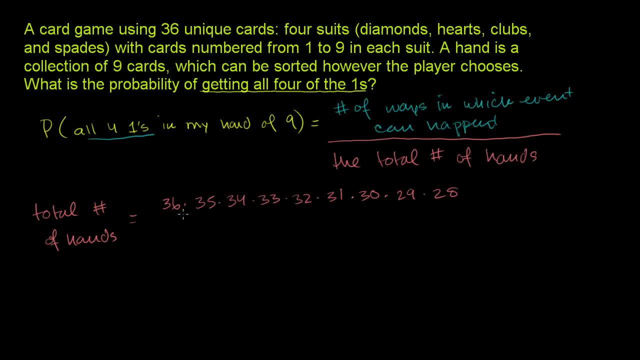 So we're over-counting here. We're over-counting for all of the different rearrangements that these cards would have. It doesn't matter whether the ace of diamonds is the first card I pick or the last card I pick. The way I've counted them right now we are counting those as. 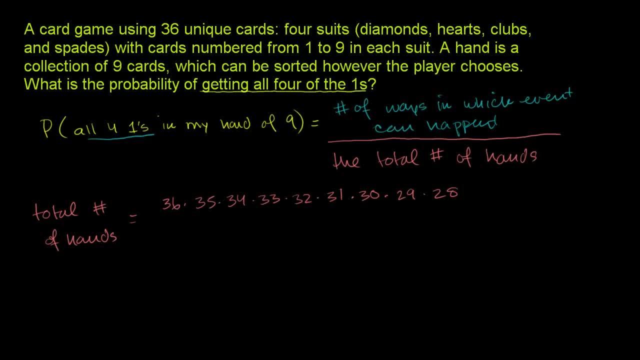 two separate hands, but they aren't two separate hands, so order doesn't matter. So what we have to do is we have to divide this. We have to divide this by the number of ways you can arrange nine things, So you could put nine of the things in the first position. 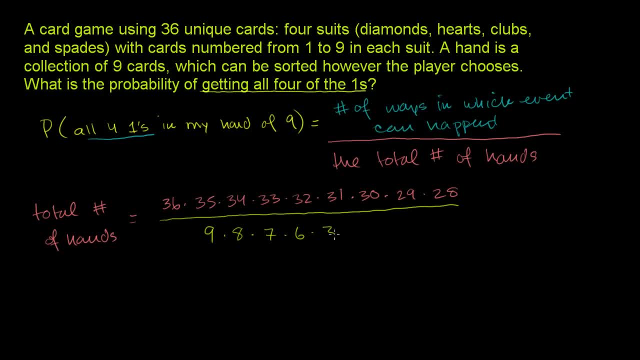 then eight in the second, seven in the third, so forth and so on. it essentially becomes 9 factorial times 2 times 1.. And we've seen this multiple times. This is essentially 36, choose 9.. This expression right here is the same thing, just so you can. 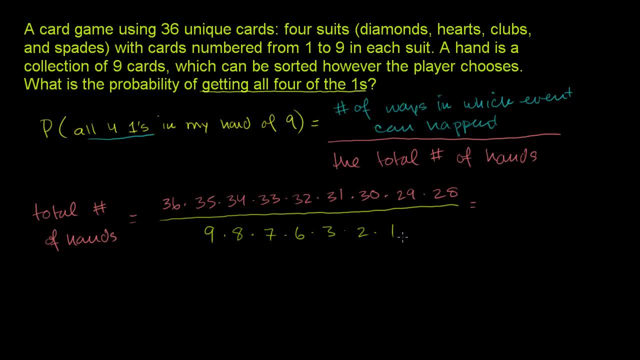 relate it to the combinatorics formulas that you might be familiar with. This is the same thing as 36 factorial over 36 minus 9 factorial. That's what this orange part is over here, Divided by 9 factorial or over 9 factorial. 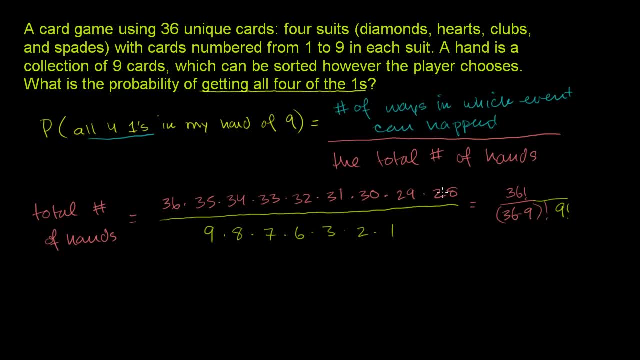 What's green is what's green, and what is orange is what's orange there. So that's the total number of hands. Now, a little bit more of a nuanced thought process is: how do we figure out the number of ways in which the event can? 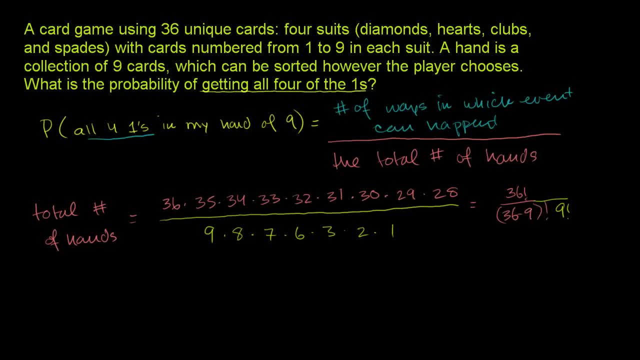 happen in which we can have all four ones. So let's figure that out. So number of ways, Or maybe we should say this: Number of hands with four ones, And this is a little bit of a thought experiment- Imagine if we were only taking four cards, if a hand only had. 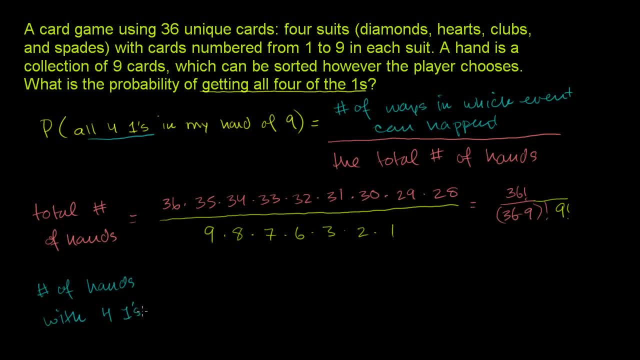 four cards in it. Well, if a card only had four hands, if a hand only had four cards in it, then the number of ways to get a hand with four ones there would only be one way, one combination. You just have four ones. 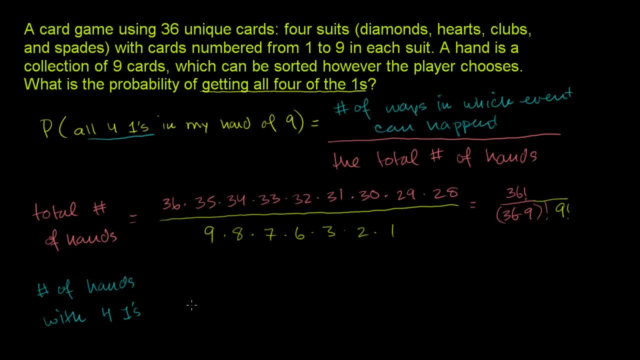 That's the only combination with four ones, if we were only picking four cards. But here we're not only picking four cards. Four of the cards are going to be ones, So four of the cards are going to be ones. I mean one, two, three, four. 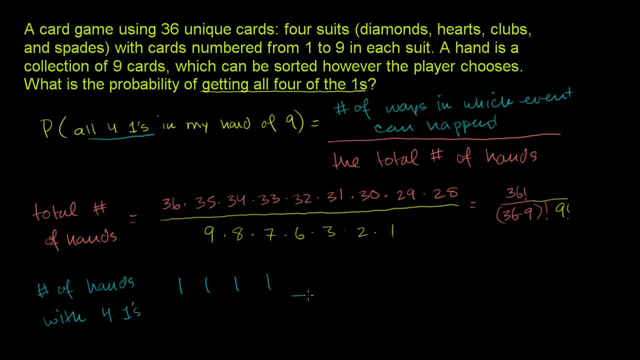 But the other five cards are going to be different. So one, two, three, four, five. So for the other five cards, if you imagine this slot, considering that of the 36, we've already we would have. we would have to pick four of them already in order for us. 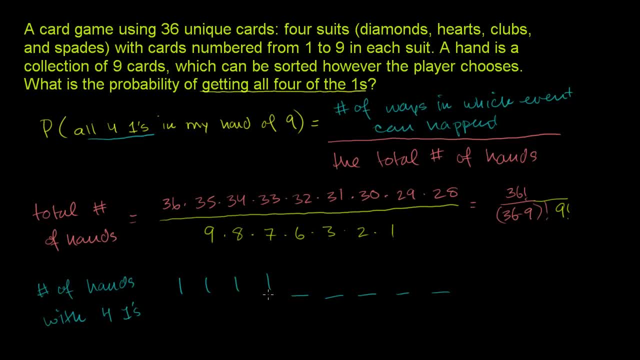 to be have four ones, So there's another if there's well, we've used up four of them. so there's 32 possible cards over in that position of the hand and then there'd be 31 in that position of the. 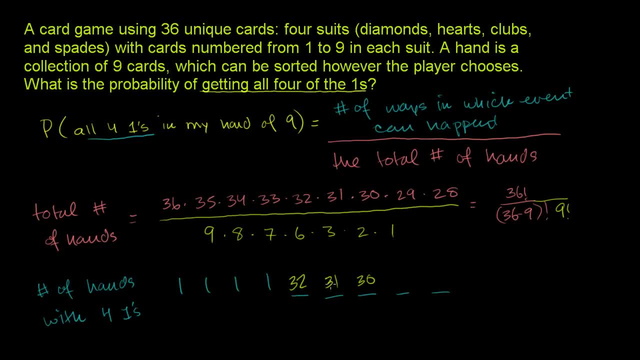 hand, and then there'd be 30, because every time we're picking a card, we're using it up, and now we only have 30 to pick from, then we only have 29 to pick from, and then we have 28 to pick from. 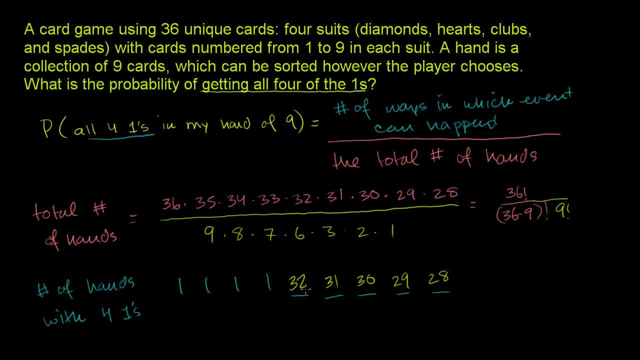 And, just like we did before, we don't have to pick four cards. We don't care about order, We don't care if we find if we pick the five of clubs first or whether we pick the five of clubs last, So we shouldn't double count it. 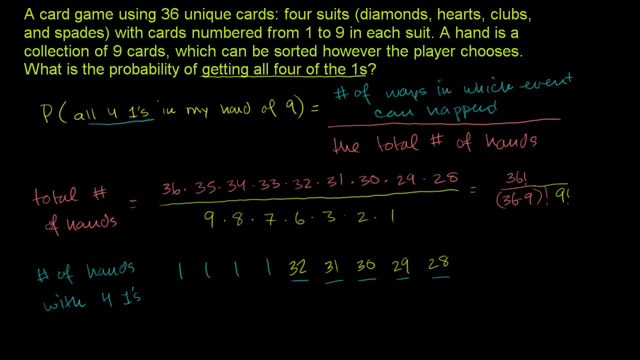 So we have to divide by the different number of ways that five cards can be arranged. So we have to divide this. we have to divide this by the different ways that five cards can be arranged. So the first card or the first position could be any. 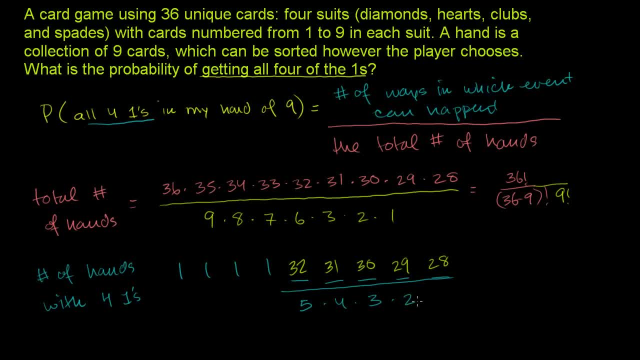 one of five cards, then four cards, then three cards, then two cards, then one cards. So the number of hands with four ones is actually is actually just this number. You're actually looking at all of the different ways you can. 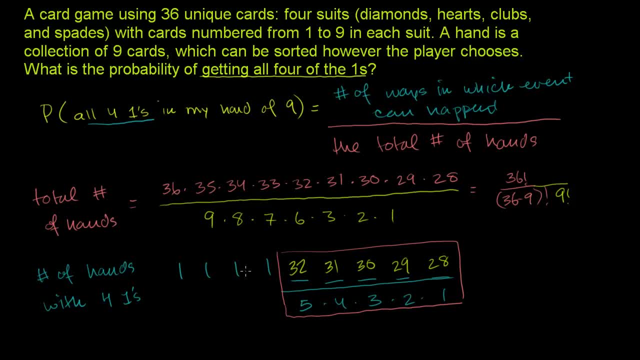 fill up the remaining cards. These four ones are just going to be four ones. There's only one way to get that. It's the remaining cards. that's going to give all of the different combinations of having four ones. So this will be a count of all of the different combinations. 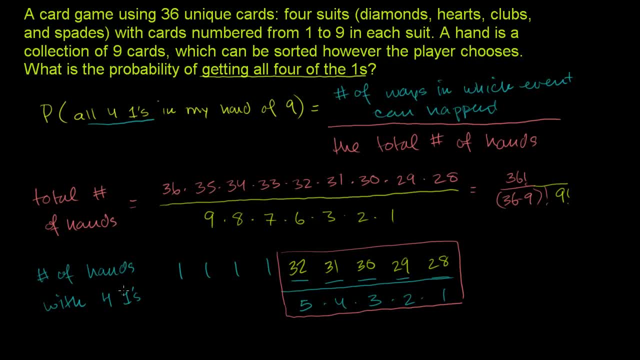 because all of the different extra stuff that you have will be all of the different hands. Now we know the total number of hands. with four ones. It's this number And now we can divide it by the total number of possible hands, and I didn't multiply them out on purpose so that we 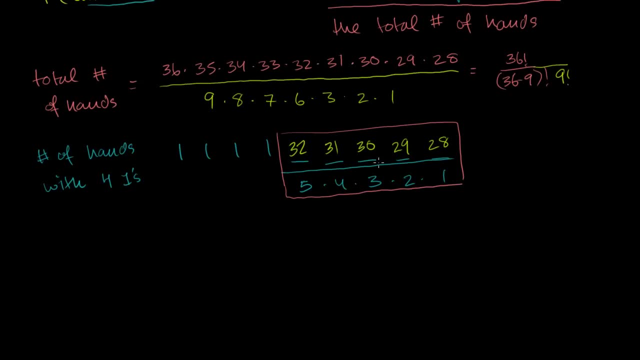 can cancel things out, So let's do that. Let's take this and divide by that. So let me just copy and paste it. Let me take that, let me copy it and let me paste it. Let's take that and let's divide it by that. 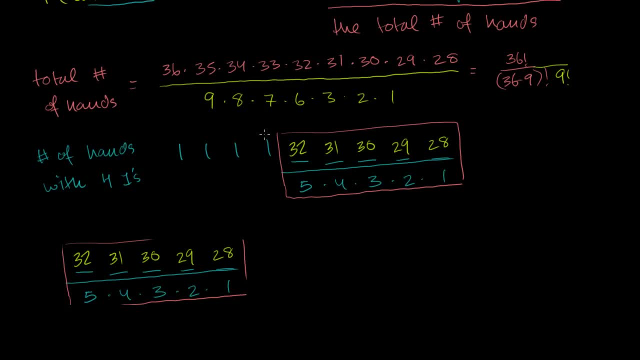 But dividing by a fraction is the same thing as multiplying by the reciprocal. So let's just multiply by the reciprocal. So let's multiply. So this is the denominator. Let's make this the numerator. So let me copy it and then let me paste it. 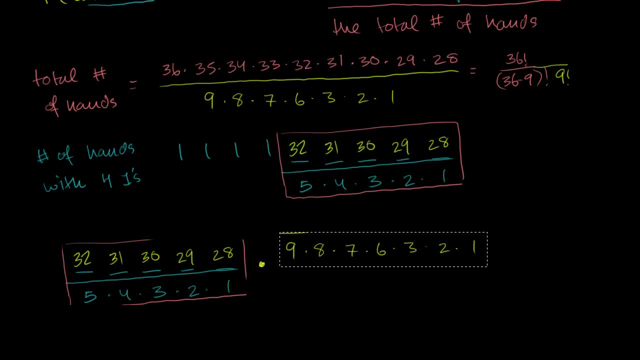 So that's the numerator And then that's the denominator up there, because we're dividing by that expression. Let me put that there. Let me get the Select tool and then let me make sure I'm selecting all of the numbers. Let me copy it and then let me paste that. 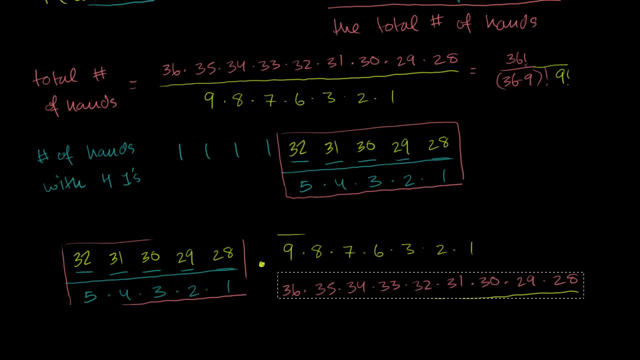 It's a little messy with those lines there, but I think this will suit our purposes. This will suit our purposes, just fine. So when we're multiplying by this, we're essentially dividing by this expression up here. Now, this we can simplify pretty easily. 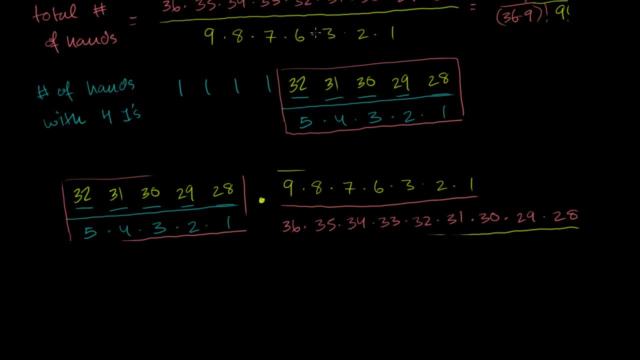 We have a- well, actually I forgot to do this should be 9 factorial. This should be 9 times 8 times 7 times 6 times 5 times 4 times 3 times 2 times 1.. So let me put that in both places. 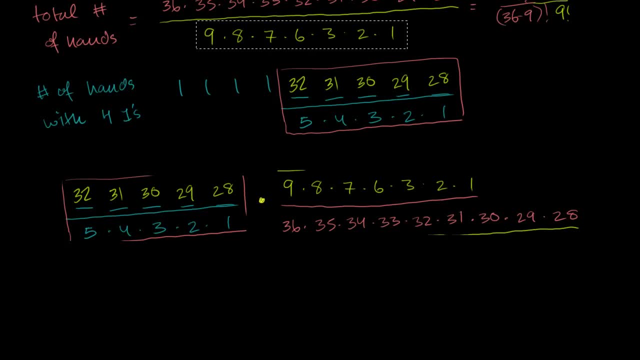 Actually, let me just clear that both places Clear. Don't want to confuse people. Clear. I'm sorry if that confused you when I wrote it earlier. This would be 9 factorial 9 times 8 times 7 times 6 times 5. 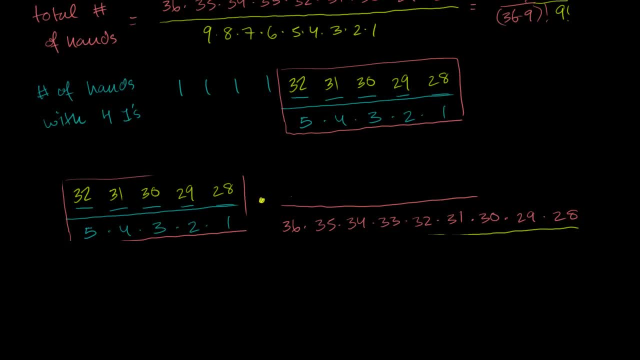 times 4 times 3 times 2 times 1.. Let me copy and paste that, now Copy, and then you paste it. That's that, right there. And then we have this in the numerator. We have 5 times 4 times 3 times 1 in the denominator. 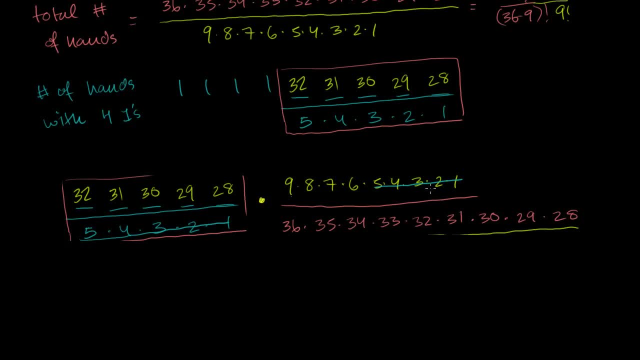 So this will cancel out with that part right over there. And then we have 32.. 32 times 31 times 30 times 29 times 28.. That is going to cancel with that That, and that cancels out. So what we're left with is just this part over here. 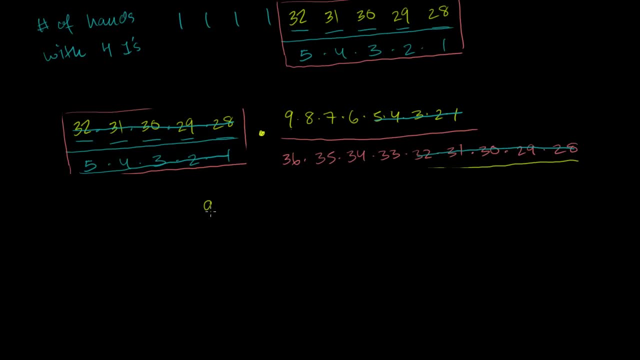 Let me rewrite it. So we're left with 9 times 8 times, 7 times 6 over- and this will just be an exercise in simplifying this expression- 36 times, 35 times, 34 times 33.. And let's see: 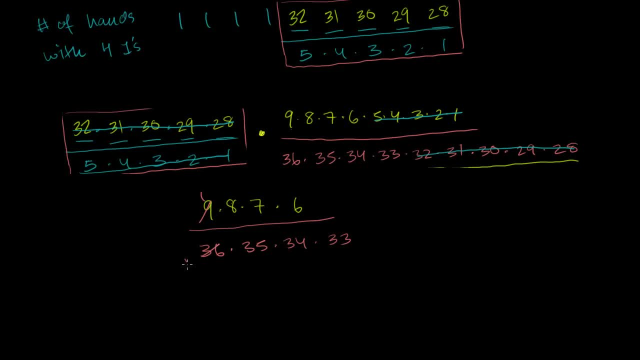 If we divide the numerator and denominator by 9,, that becomes a 1. This becomes a 4. You can divide the numerator and denominator by 4.. This becomes a 2. This becomes a 1.. You divide numerator and denominator by 7.. 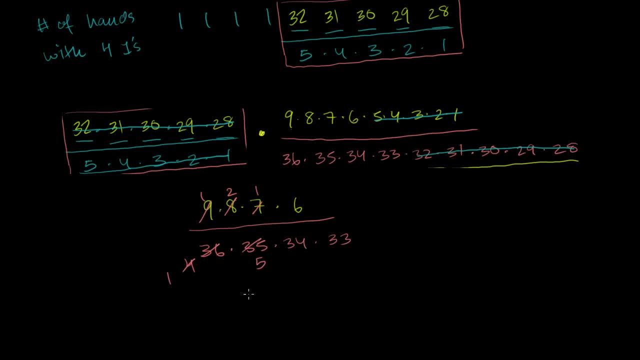 This becomes a 1.. This becomes a 5.. You can divide both by 2 again, and then this becomes a 1.. This becomes a 17. And you could divide this and this by 3.. This becomes a 2.. 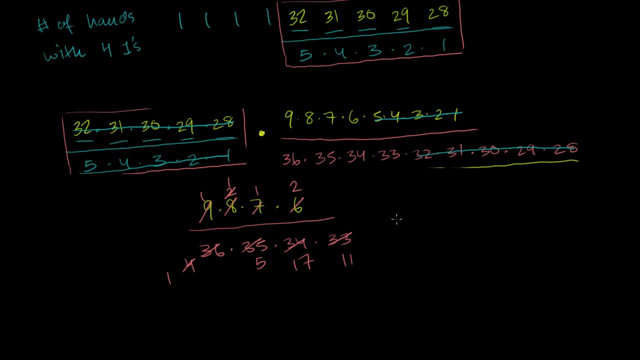 And then this becomes an 11.. So we're left with the probability of having all four 1's in my hand of 9 that I'm selecting from 36 unique cards is equal to in the numerator. I'm just left with this 2,. 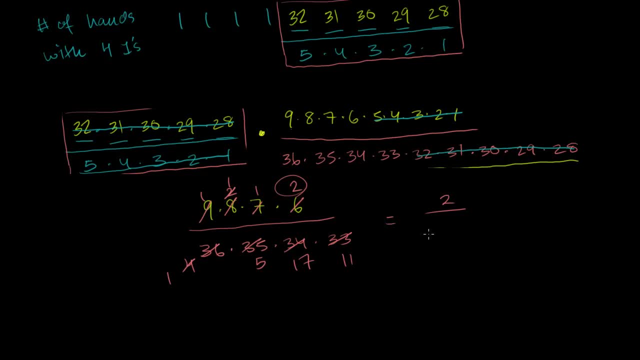 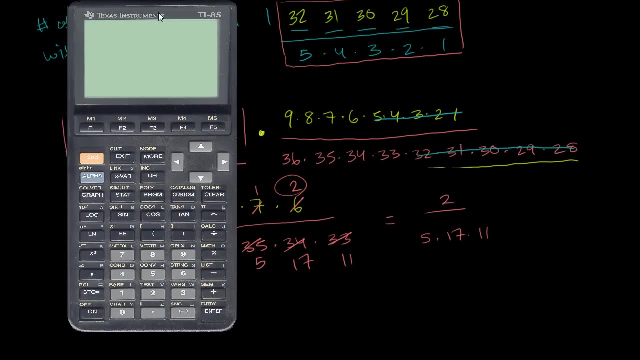 times 1, times 1, times 1.. So it's equal to 2 over 5 times 17 times 11.. And that is drum roll. this was kind of an involved problem. 5 times 17 times 11 is equal to 935.. 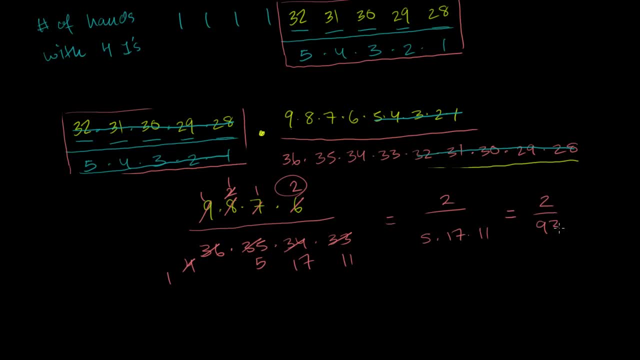 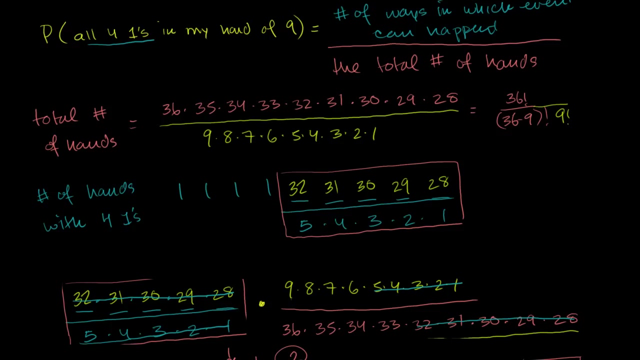 So it's equal to 2 over 935.. So about roughly 2 in 1,000 chance or 1 in 500. roughly speaking, this is the exact odds. you have roughly 1 in 500 chance of getting all 4 of the 1's in your hand of 9 when 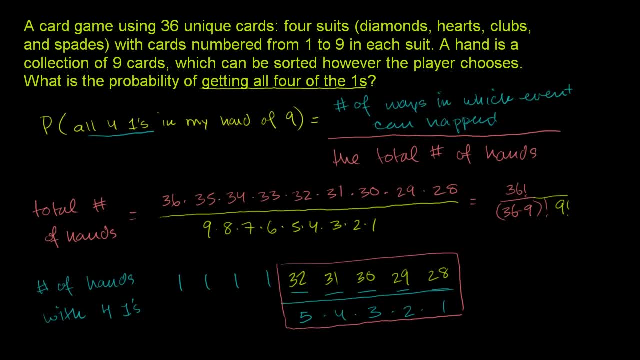 you're selecting from 36 unique cards. Thank you.